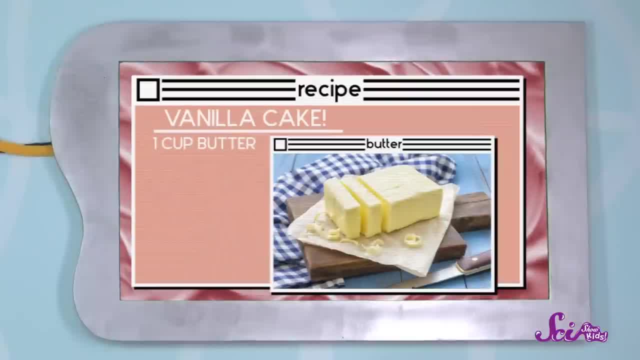 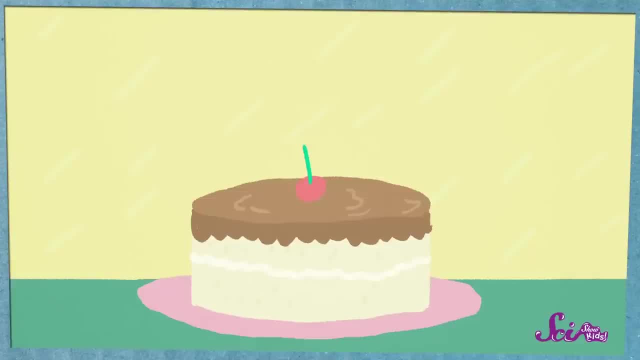 Next is butter, which we're using as the fat for our cake. Now, when we say fat, we don't mean the fat that we have on our bodies. We're talking about a type of food. You already know that this cake is going to be made up of all the ingredients in our recipe. 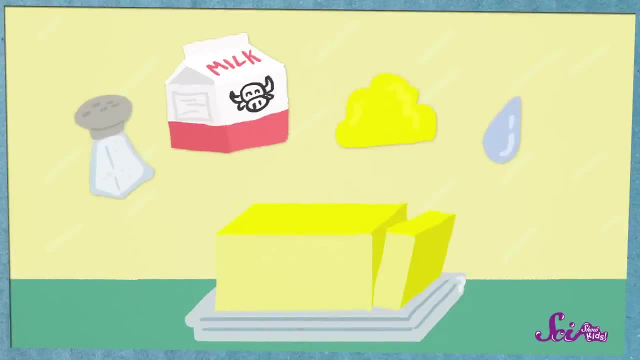 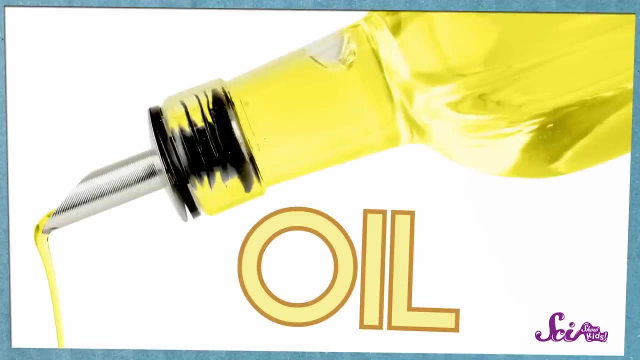 Butter is one of them, But butter is made of its own list of ingredients too, And fat is one of them. Lots of food have fat in them, like oil, which some recipes use instead of butter. No matter what form of fat you're using, the fat's job is to coat the food. 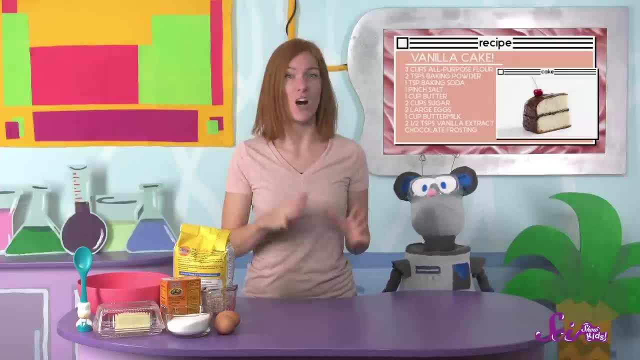 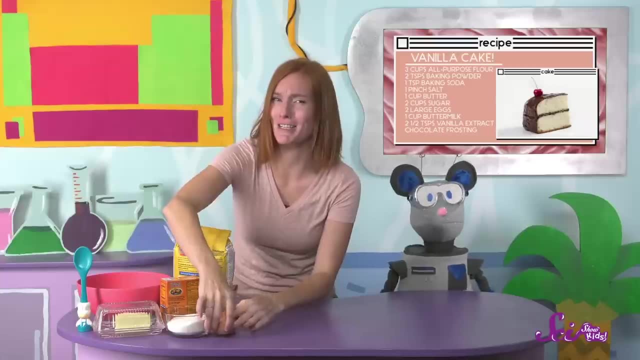 So butter is one of them, And flour, which keeps it from mixing with the water too much. That will make our cake soft and fluffy. Most recipes use eggs too, for a few different reasons. Our recipe calls for two eggs. 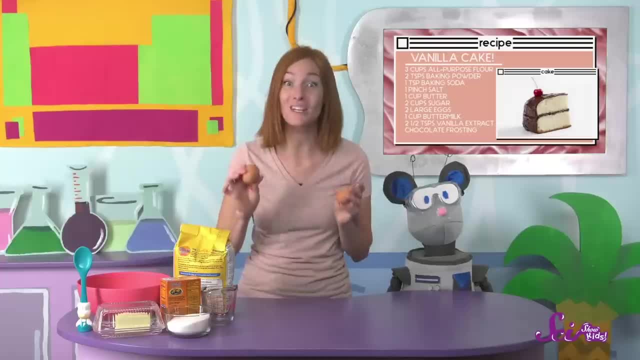 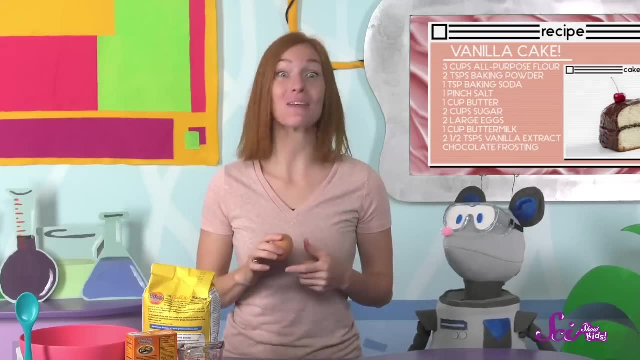 Eggs are fun to crack, but make sure a grown-up is helping you. One of the things eggs do is help turn the batter from a liquid into a solid cake once it's in the oven, And they can also help the cake rise. Whipping egg whites will fill them with air bubbles. 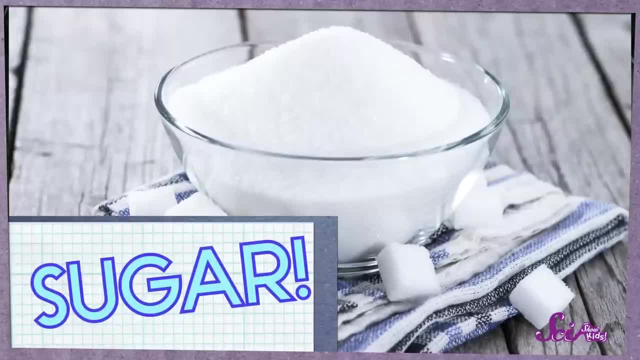 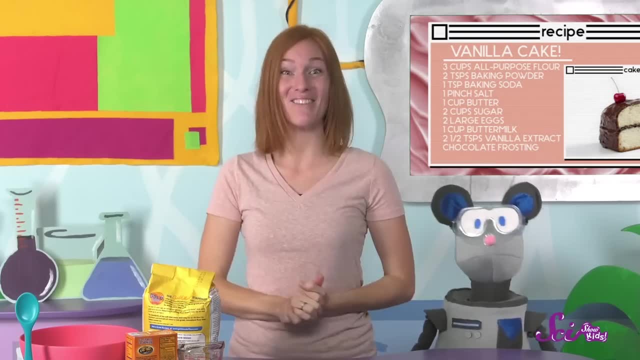 That air will help the cake rise. We're also using sugar in our recipe, and I bet you can guess why It'll make the cake taste terrific, and I can't wait. Alright Squeaks, let's put all of the ingredients together and put our cake in the oven. 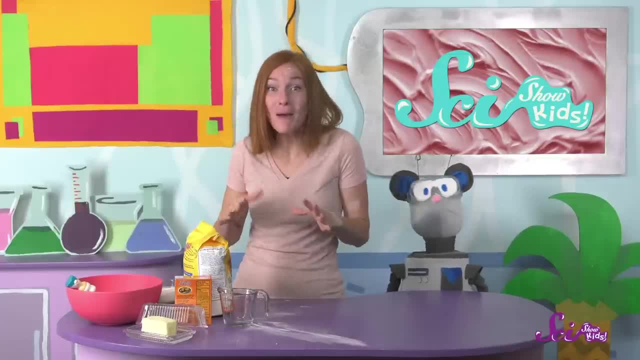 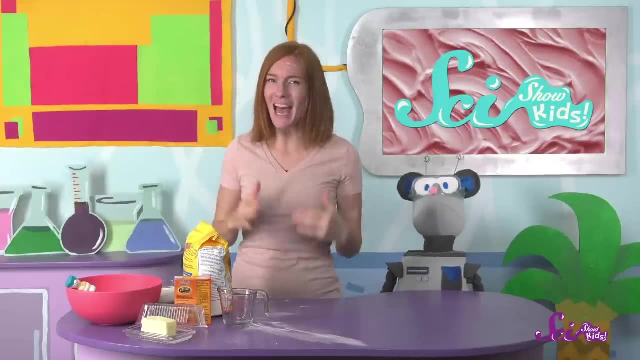 Our cake has been baking in the oven for a little while now. We measured everything perfectly, so our flour, butter, baking soda, eggs and all the other ingredients are reacting to each other. to turn the batter into a solid cake, We're going to need a little bit of butter. 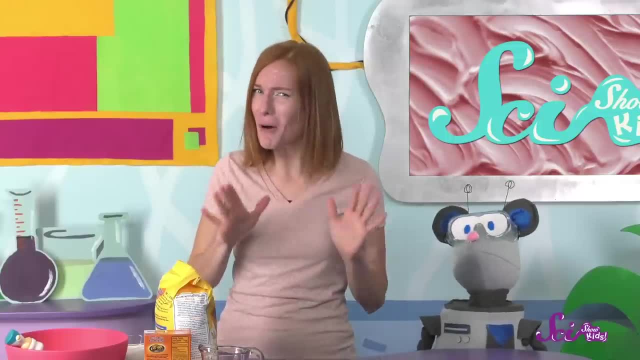 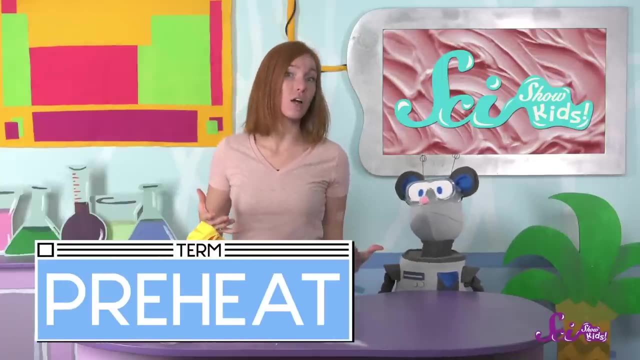 We're going to need a little bit of flour. We're going to need a little bit of butter. We've set a timer so we know when it's done baking, and it should be any minute now. We also preheated our oven earlier, which means we turned it on before we started our 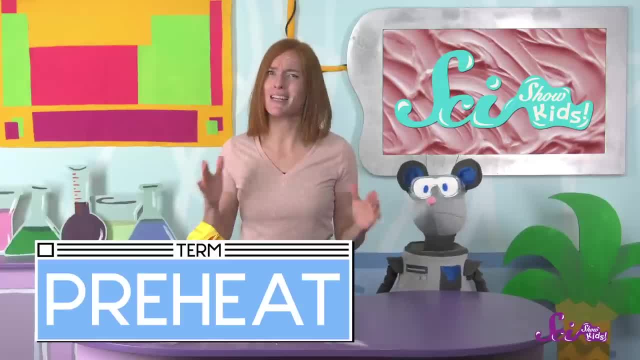 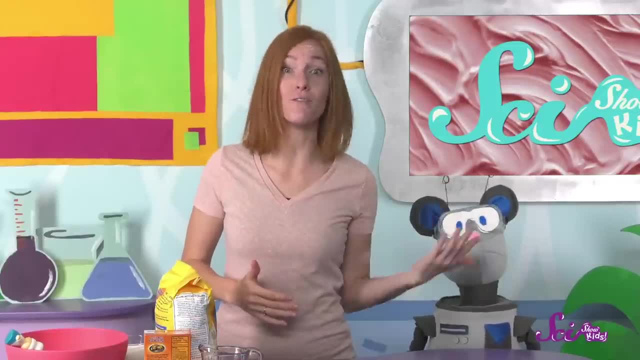 project because the oven takes some time to warm up and it needs to get very, very hot in there. Right now our oven is at 175 degrees Celsius or 350 degrees Fahrenheit. That means it's more than hot enough for all those bubbles in the batter to get bigger. 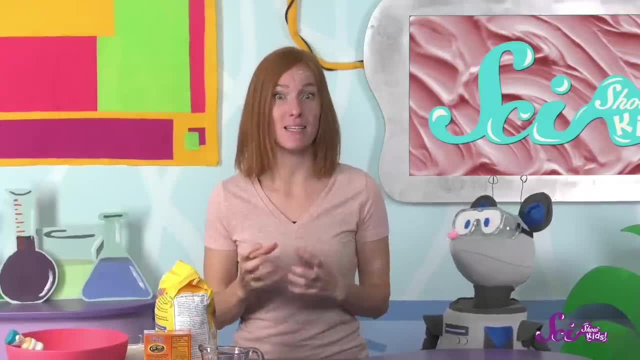 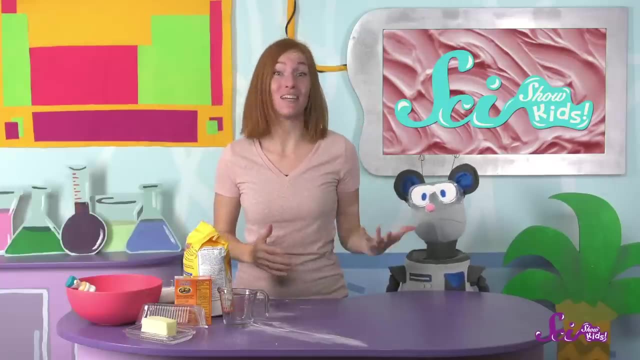 helping it rise. Other ingredients are breaking down and mixing to make yummy flavors, while the eggs and the flour help hold it all together. Baking is a great activity for kids and grown-ups to do together, but using the oven preheating.